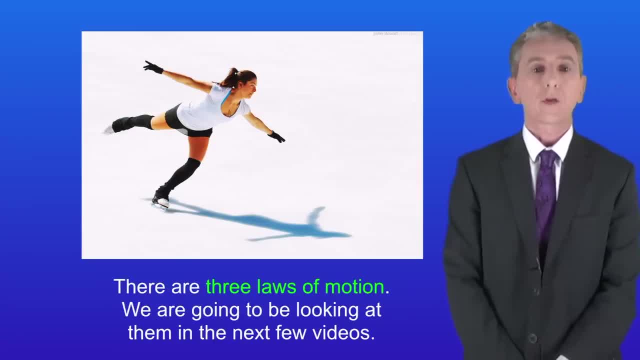 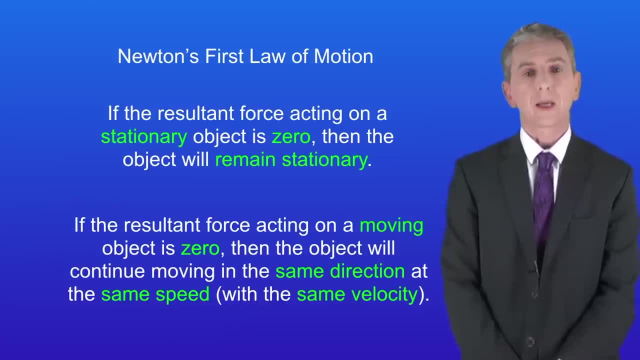 effects that forces have on the motion of an object. There are three laws of motion and we're going to be looking at them in the next few videos. I'm showing you Newton's first law of motion here: If the resultant force acting on a stationary object is zero, 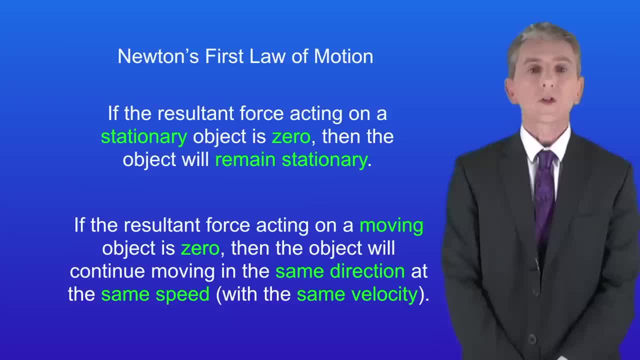 then the object will remain stationary. If the resultant force acting on a moving object is zero, then the object will continue moving in the same direction at the same speed, In other words with the same velocity. Now this looks a bit tricky, but I promise you it's easier than it looks. I'm showing. 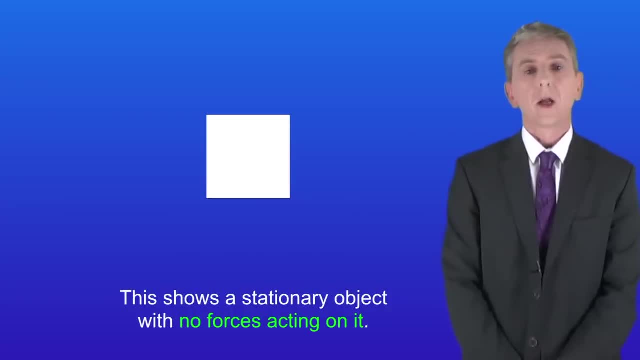 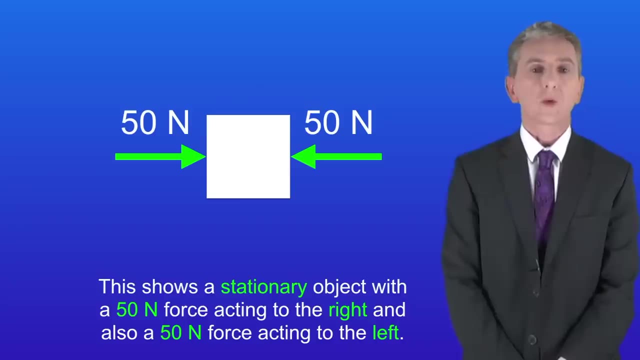 you here a stationary object with no forces acting on it. Because there's no resultant force, the object will remain stationary. This shows a stationary object with a 50 Newton force acting to the right and also a 50 Newton force acting to the left, In this case the 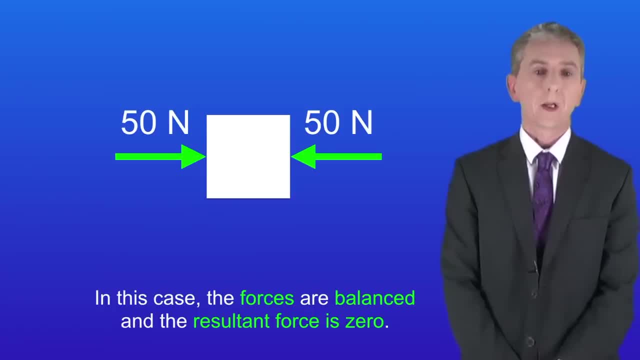 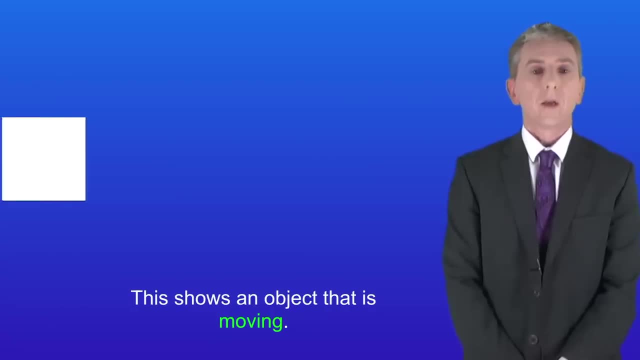 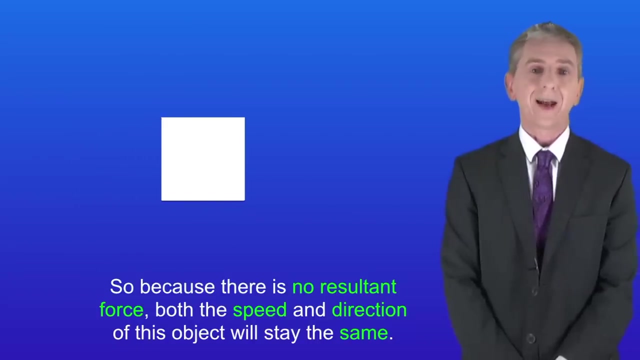 forces are balanced and the resultant force is zero. So, once again, this object will remain stationary. OK, now this shows an object that's moving. There are no forces at all acting on this object. So, because there's no resultant force, both the speed and direction of this object. 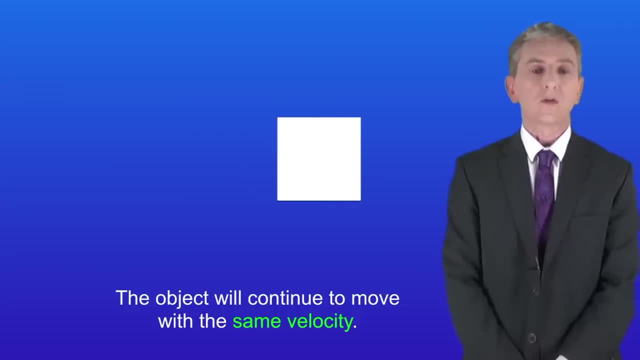 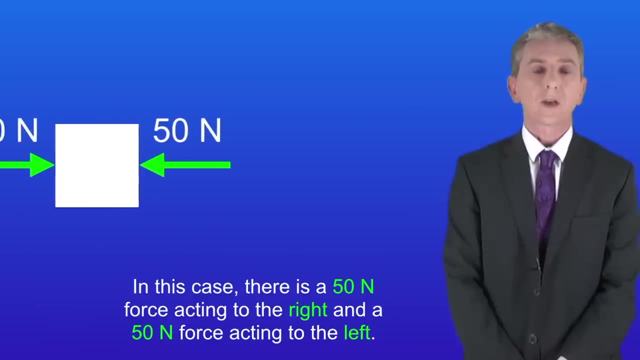 will stay the same. In other words, the object will continue moving at the same velocity. This shows another object that's moving. In this case there's a 50 Newtons force acting to the right and the 50 Newton force acting to the left, Because the forces are balanced. 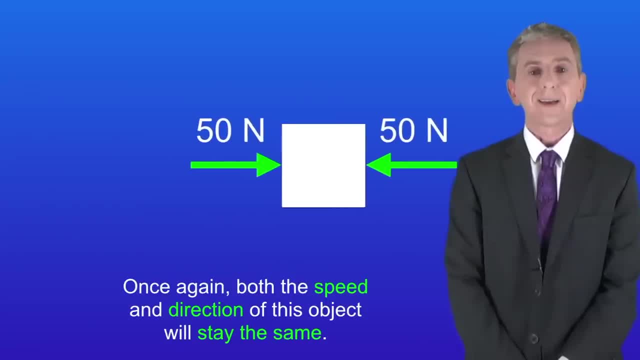 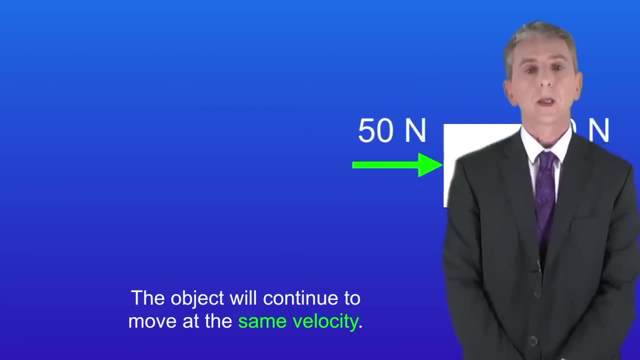 the resultant force is zero is zero. So, once again, both the speed and direction of this object will stay the same. The object will continue to move at the same velocity. So the key fact is that the velocity of an object will only change if a resultant force 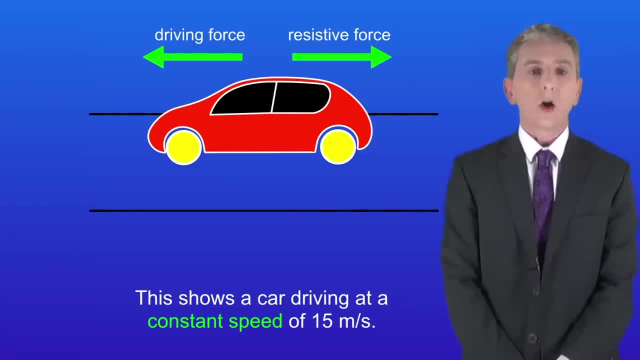 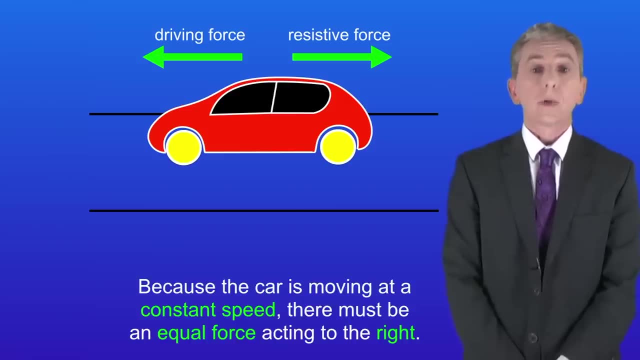 is acting on the object. I'm showing you here, a car driving at a constant speed of 15 metres per second. The driving force of the engine is acting to the left. Because the car is moving at a constant speed, there must be an equal force acting to the. 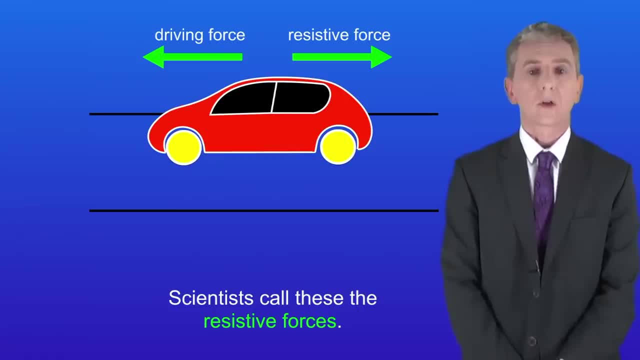 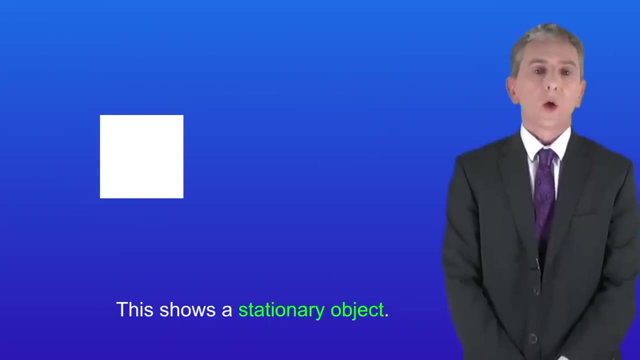 right. Scientists call these the resistive forces. The resistive forces include friction with the air and also friction with the road. Ok, so let's look now at what happens when a resultant force acts on an object. This shows a stationary object. We're applying a resultant force of 50 Newtons.